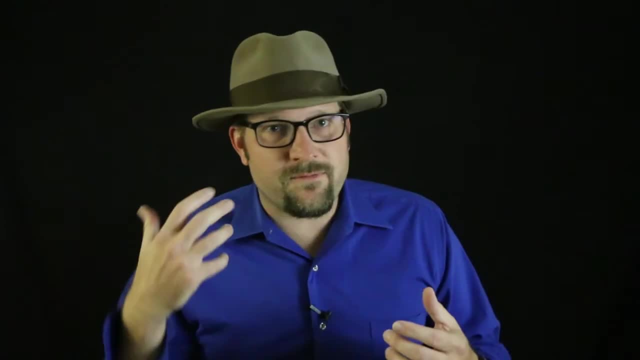 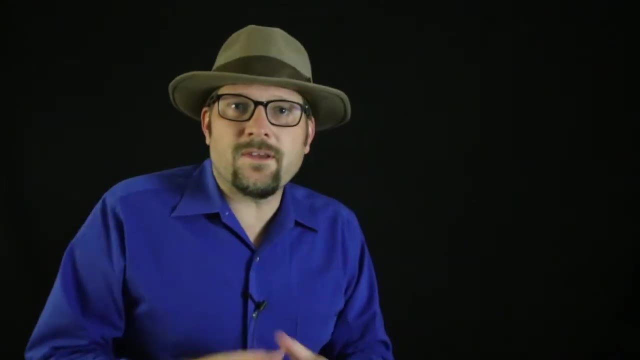 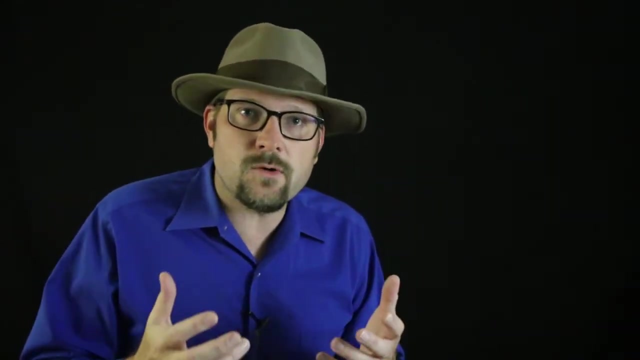 into lineages that would go on to evolve into modern amphibians, the list amphibia, as well as reptiles, birds and mammals, the amioda. During the early Mississippian period, a handful of early tetrapods were exploiting the shallow rivers and ponds using their forelimbs mostly. 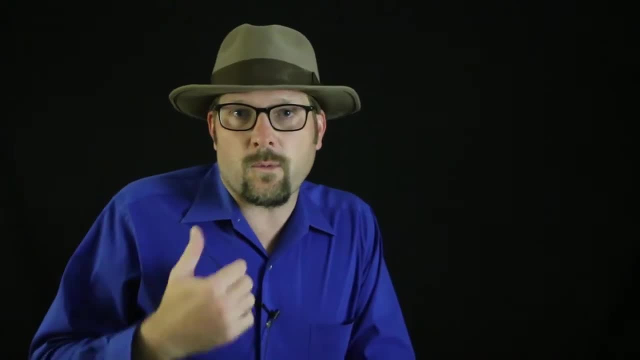 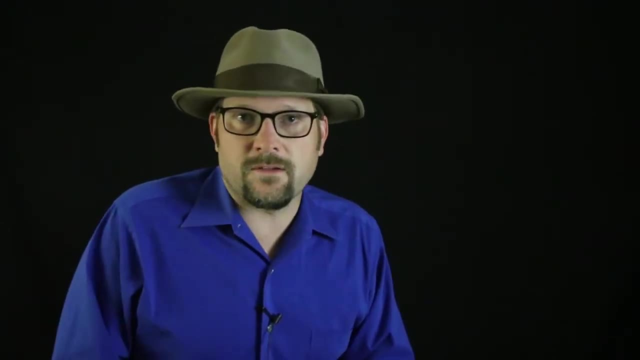 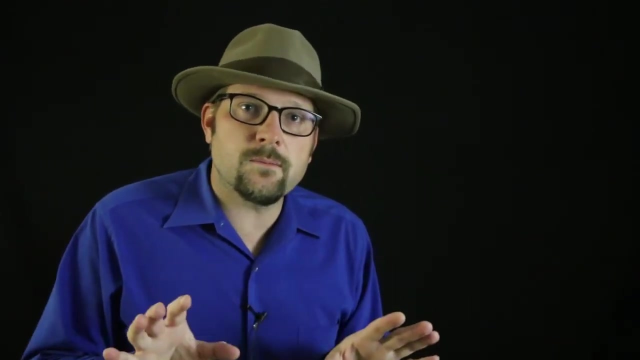 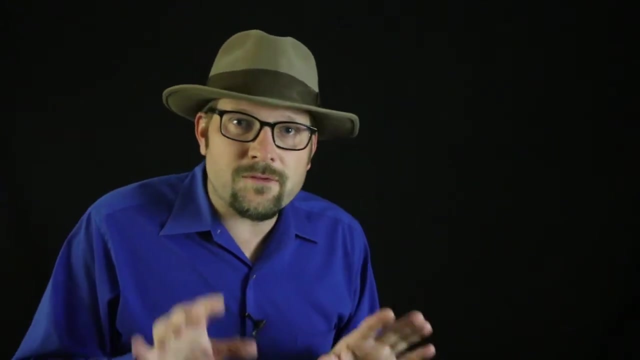 for swimming with limited abilities for walking short distances. These limbs likely functioned in emergency situations when the shallow ponds or rivers would dry up during the summer seasons. These limbs would allow these early tetrapods to escape the drying up of pools of water and be able to find a new home and survive to reproduce. 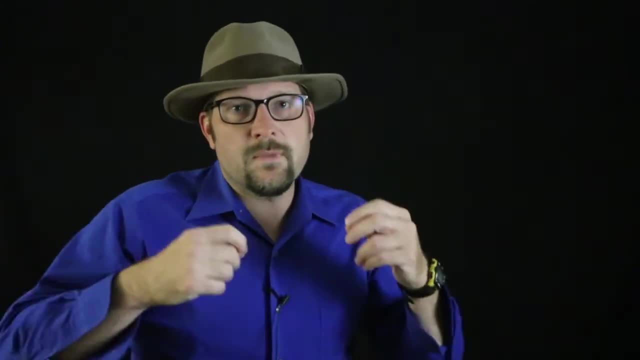 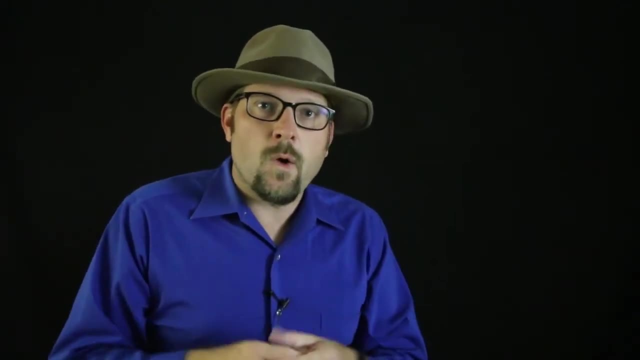 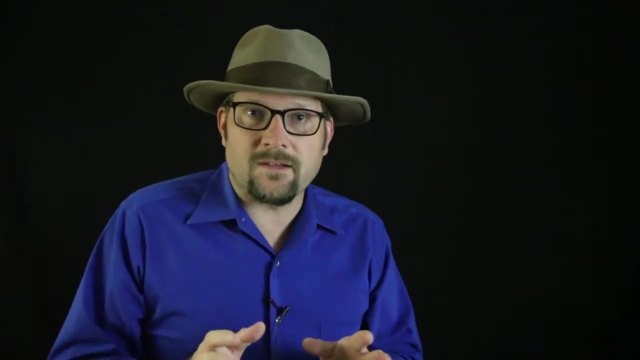 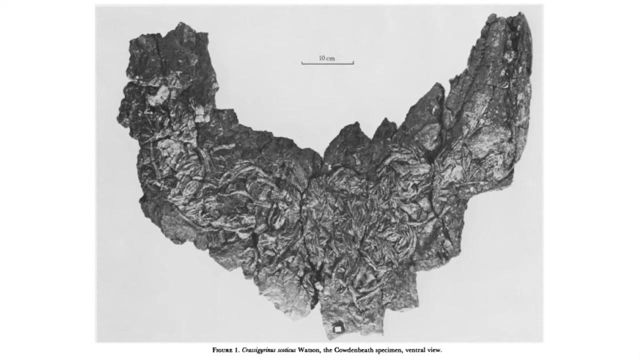 As such, most of the early Mississippian tetrapods were spending most of their life cycle in the water. One of the best known early Mississippian tetrapods is Crassiogyrus from Scotland. Crassiogyrus was about the size of a medium crocodile, about 1.5 meters. 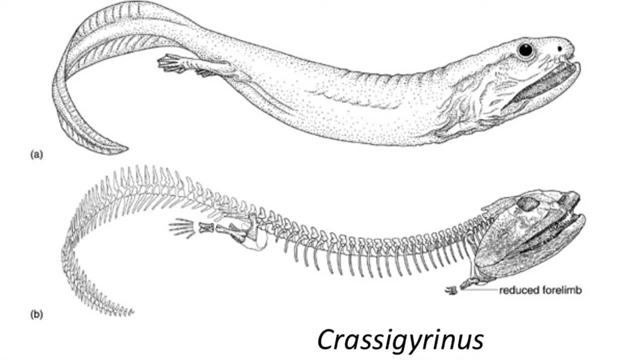 long, with a skull that measured about 38 centimeters long. The head was large and these creatures were likely feeding on fish. The weird thing about Crassiogyrus was that it had a very reduced forelimb With a very small head. it could easily be found in the 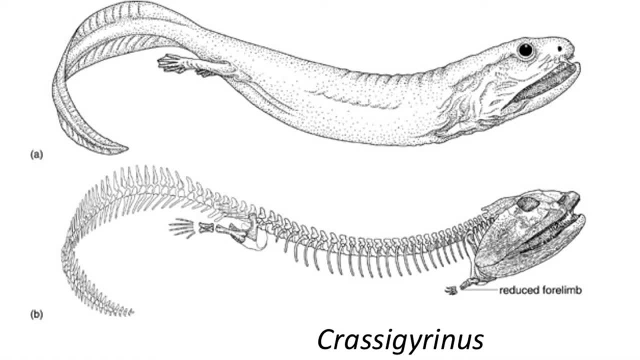 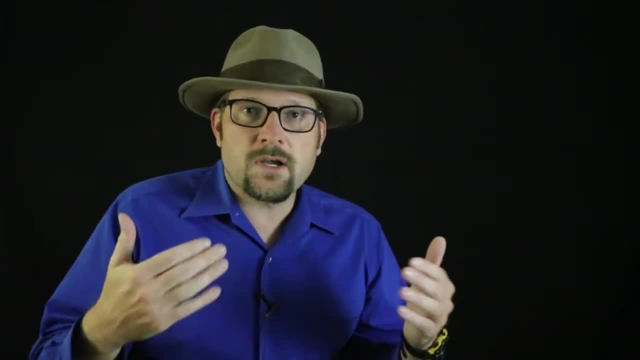 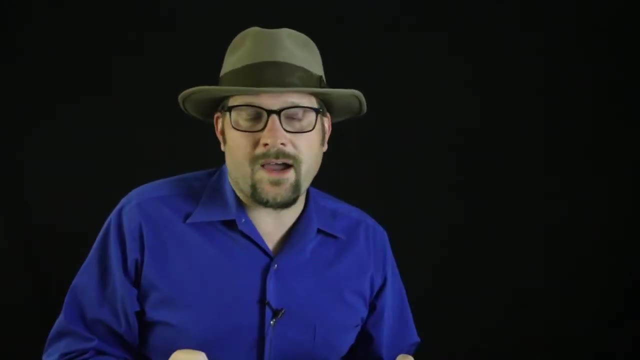 water with a small little dainty hand. The posterior limbs were better developed, but much of the locomotion of this creature was powered by a large, compressed tail. Such anatomy likely meant that the animal spent a great deal of time in the water. 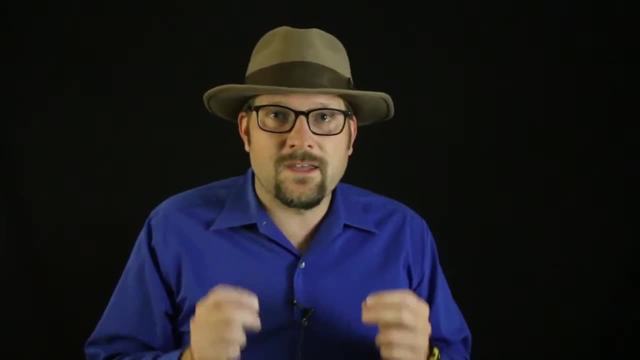 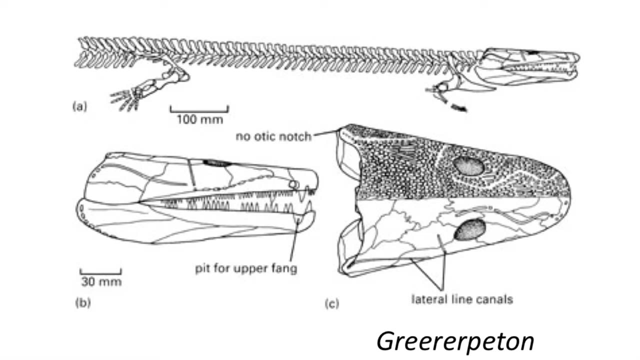 Another early vertebrate from the early Mississippian is Giriaptrion from West Virginia. It too was a fairly large tetrapod With lengths up to 3.5 meters long. it could be found in the water. Bony scutes covered the body which made this creature armored, which is 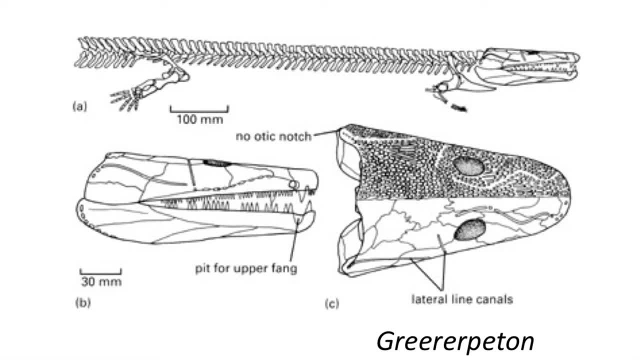 not found in modern amphibians. The body was extremely elongated, with numerous vertebrae between the forelimb and the hindlimb, such that it resembled a long snake. The tail was also compressed, which meant that it was used for swimming by moving it backward and forward. 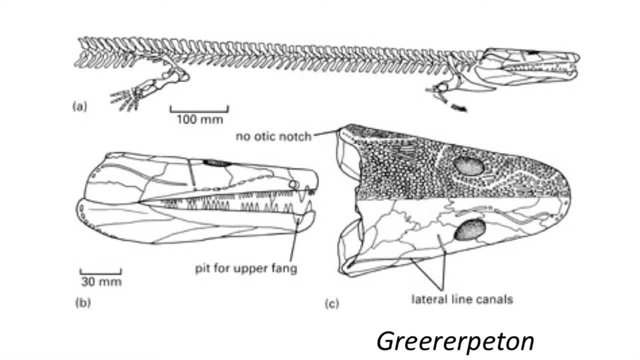 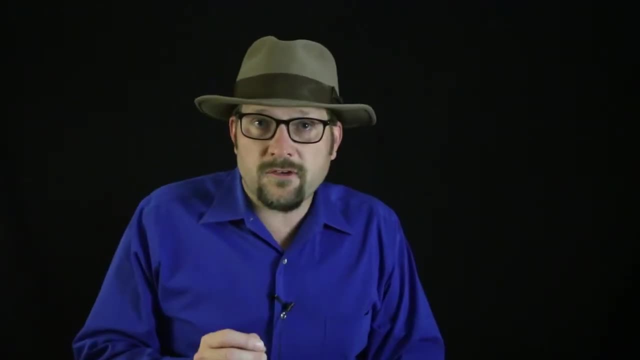 The skull was flattened and lacked an otic notch, With the bones grooved with lateral line canals that served to detect movement and vibrations in the surrounding water. Giriaptrion was likely feeding on fish primarily. One of the innovations we see in these early tetrapods is improvement in jaw muscles, which 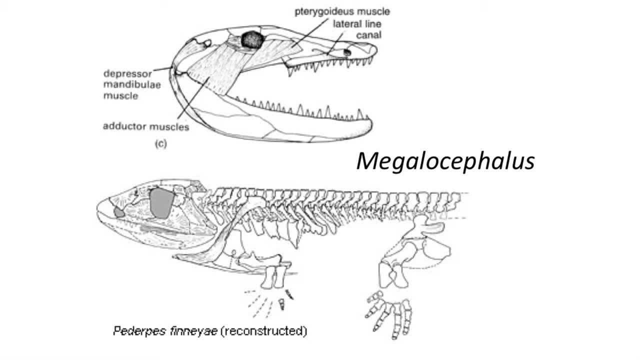 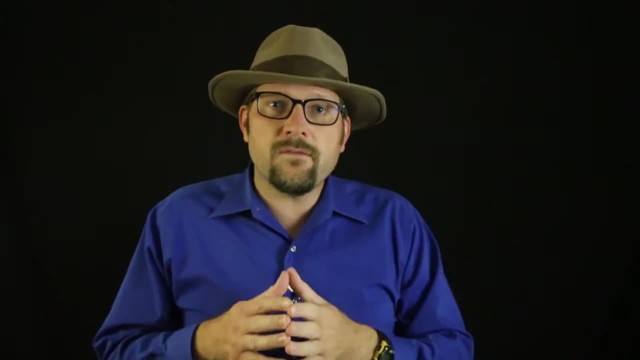 is found in the Mississippian tetrapod Megaleocephalus, which provided a stronger bite as well as muscles to open the jaw. Now, many of these early tetrapods are placed in a large group of early tetrapods called 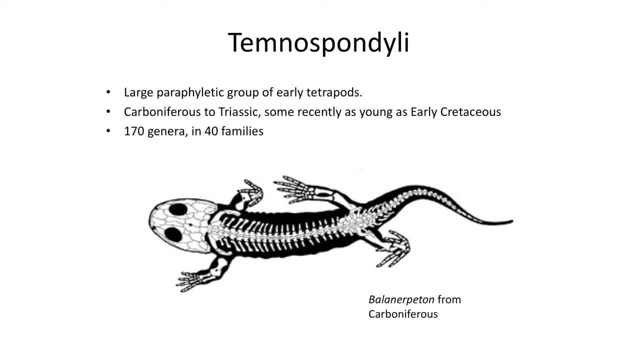 Temdospundylans, which is a large paraphyletic group of early tetrapods which include over 170 genera and 40 families. The Temdospundyla were a successful group of basal tetrapods that survived into the Mesozoic, as recently as the early Cretaceous. 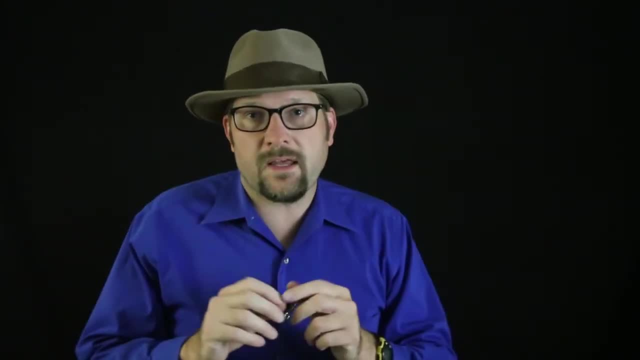 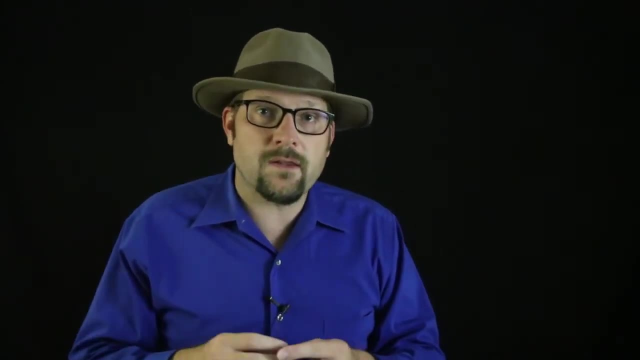 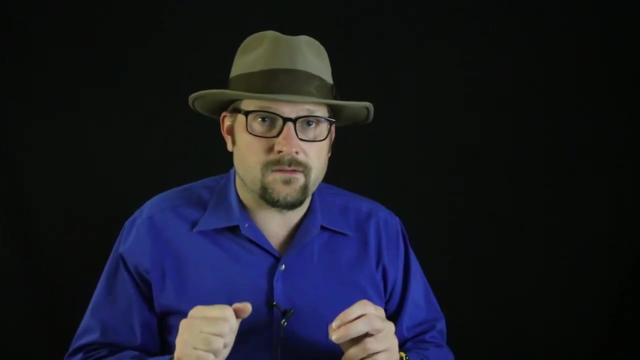 Next few fossils I'll talk about belong to a monophyletic branch called the Eutemnospundyla, which includes a very diverse group of late Paleozoic, early tetrapods, as well as the lineage that leads to modern list amphibians like frogs and salamanders. As such, this 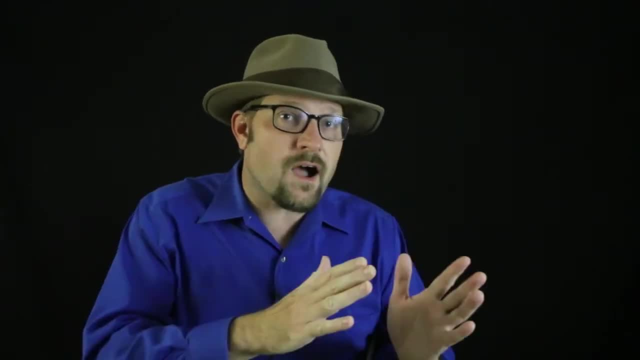 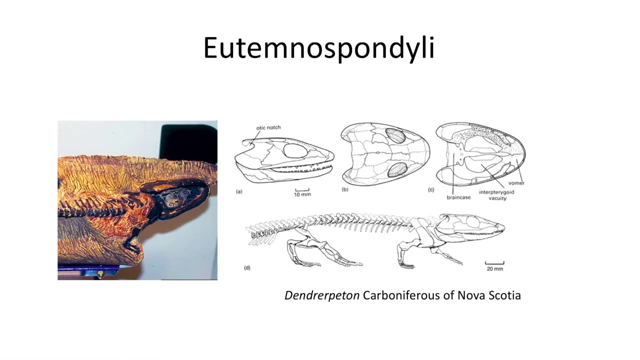 group is considered more closely related to frogs than to lizards. One of the best known Eutemnospundylans is from the fantastic Joggings fossil site in Nova Scotia, a Pennsylvania site in Canada. This is Dendoropteron. What is so amazing? 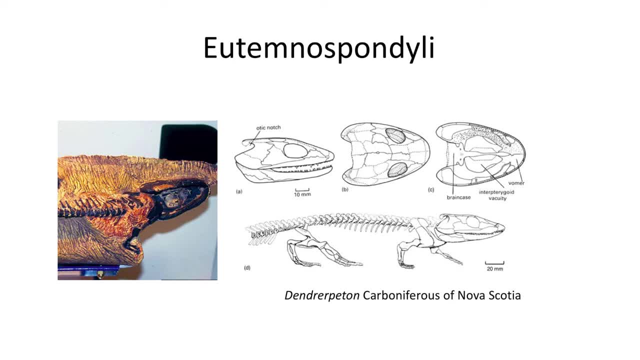 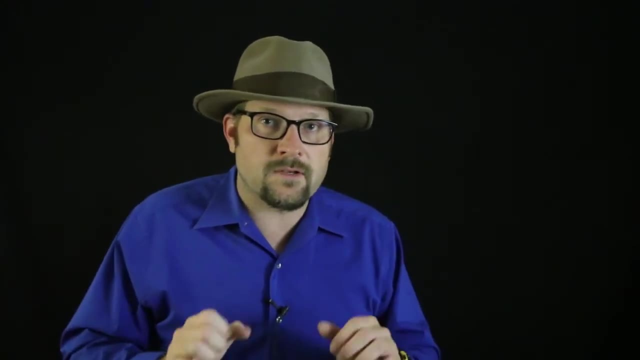 about Dendoropteron is that it is much more of a terrestrial animal than we have seen so far in this class. Dendroptes- Dendroptes, Dendroptes- hollow, petrified lochiopsid trees that are found along the modern day coastline. 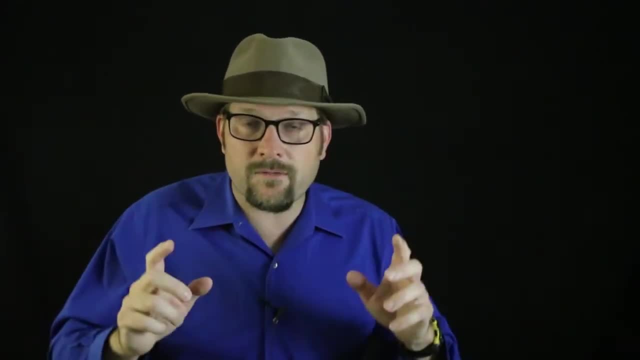 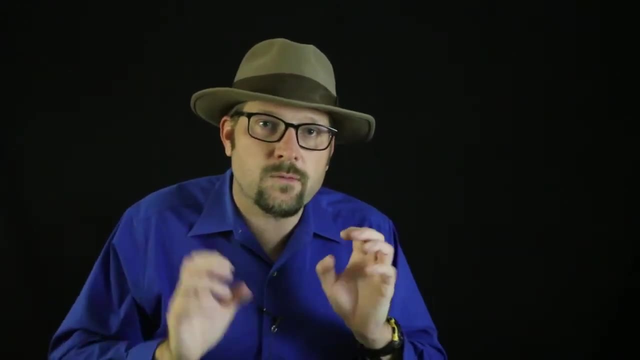 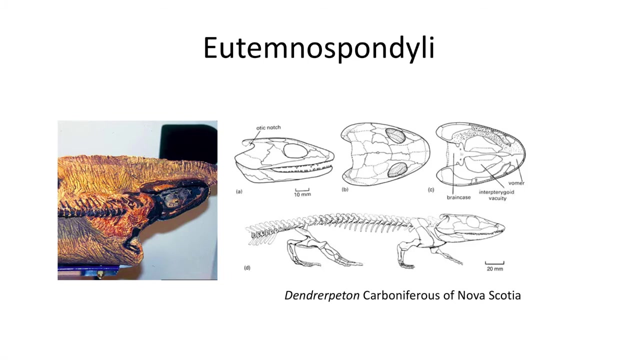 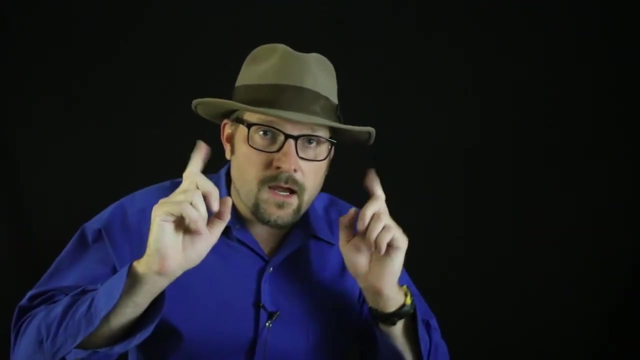 Dendriopteron could climb out of the river and into and on trees, so they are the first tetrapod that could start climbing around. We can see that they have much more upright bodies with a more rounded head. The otic notch contains a stapes, so they could hear in the air and likely were feeding. 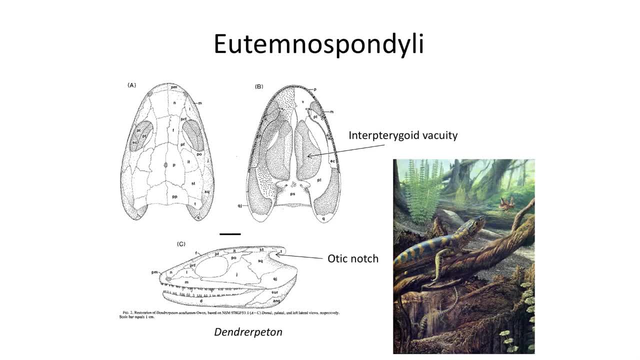 on insects rather than fish. As such, they had large eyes and they have a large interterygoid vacuity, which is an opening in the roof of the mouth, a trait found in other advanced eutendospondylans. 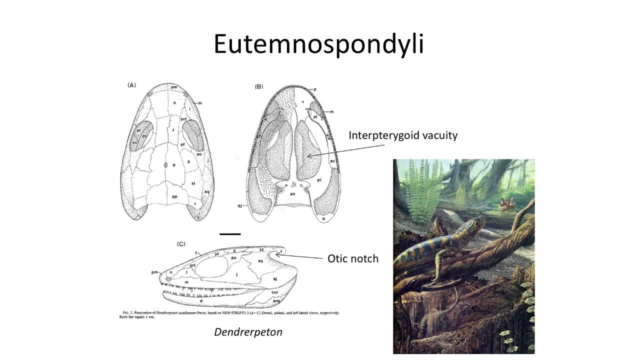 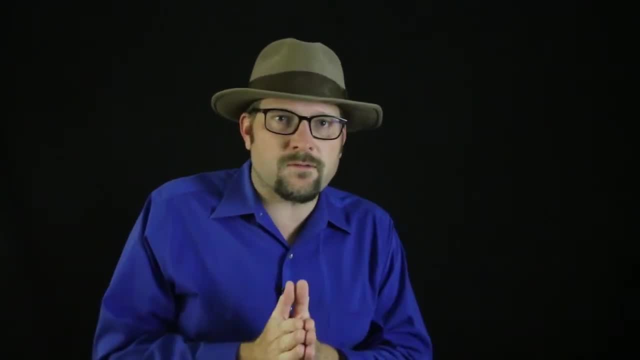 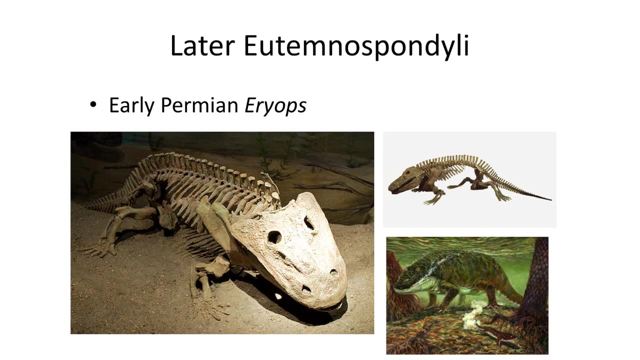 The vulmar bone is also large in the roof of the mouth. During the Permian and even into the Triassic, The eutemnospondylans were very successful. The Permians saw the origin of some very large groups, including the giant Uriops. 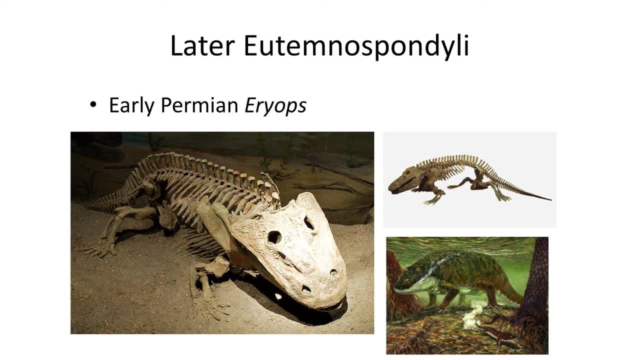 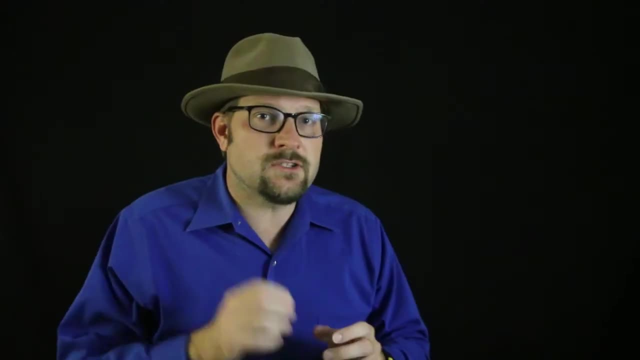 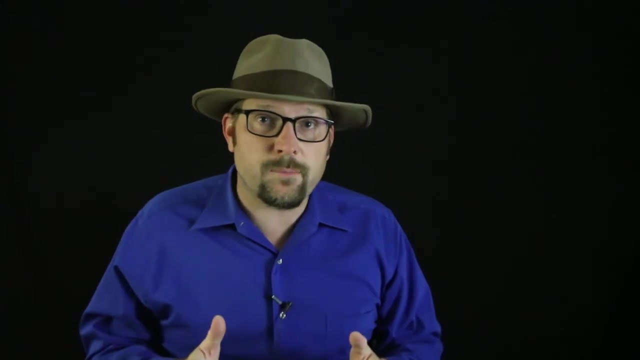 Known from Texas, which grew to be about 2 meters long. These groups were most closely related to modern amphibians. As such, some of these forms show a unique lifestyle of delaying the development of adult features And retaining juvenile life. This variability in the development of traits during the lifespan is referred to as heterochrony. 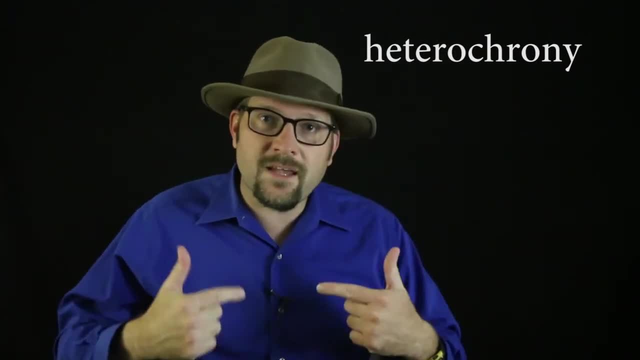 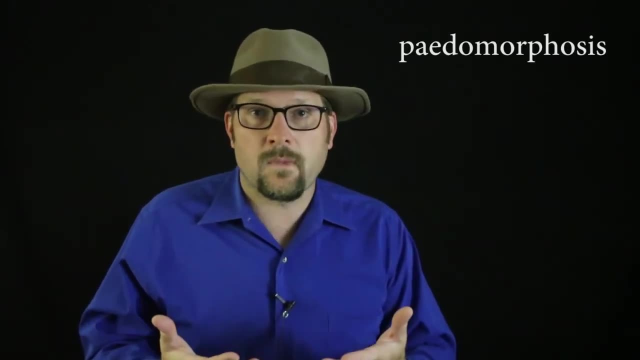 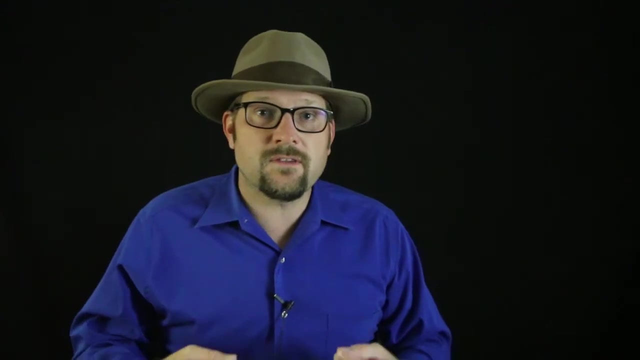 which means different timing. The retention of juvenile traits like gills into adulthood is referred to as pedomorphism, While paramorphism refers to the expansion of characters late in life, such as the ossification of the genitalia. It also refers to the expansion of the pelvis and carpals and tarsals, the finger and toe. 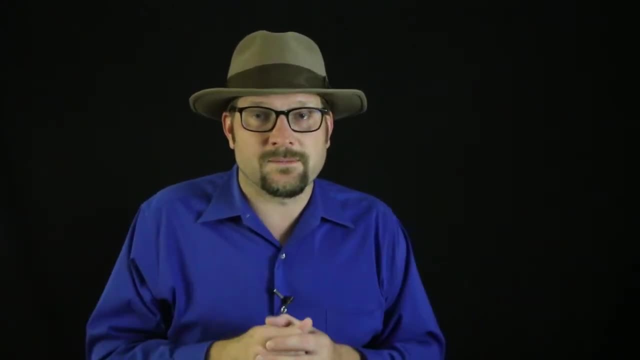 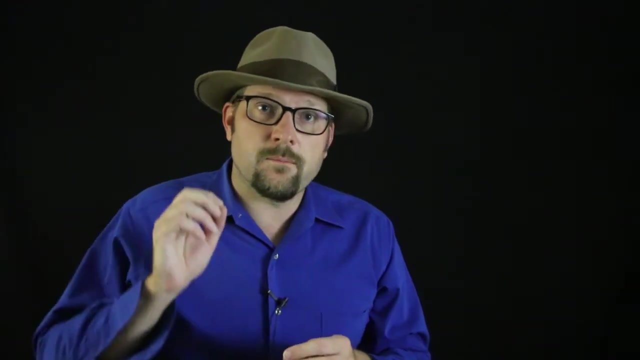 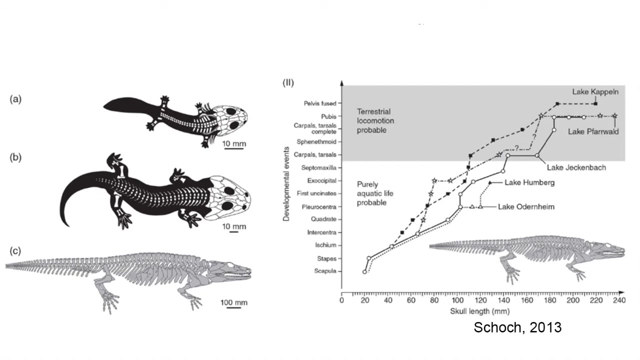 bones to facilitate terrestrial locomotion. We see this heterochrony play out with the eutemnospondylans in the Pennsylvania and Permian, fossils of Sclerocephalus and Orthocantalus in Germany. Now here a large series of fossil individuals have been found from different ancient lake. 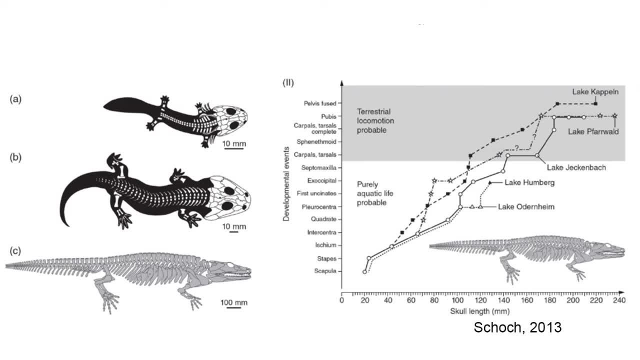 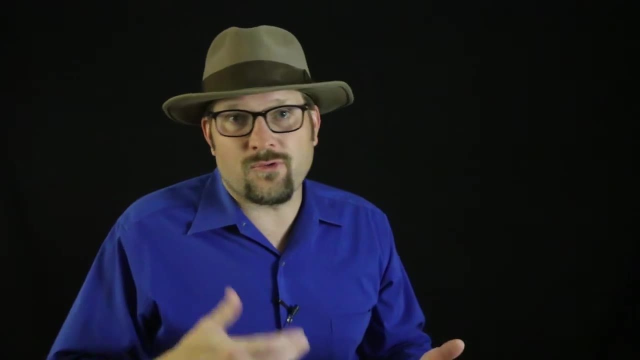 systems, Showing how, in some lakes, juvenile forms are the only ones found, while in other lakes, the same genre shows more advanced adult features which allowed them to move out of the aquatic habitat. if the lake was prone to drying out or the presence of aquatic predators, that they needed to escape from. We see such patterns in modern salamanders and frogs, where juvenile forms can become sexually mature. The eutemnospondylans are the only ones that can survive in the water and never take to the land and spend the entire life span in the water. Within these eutemnospondylans, we begin to see the development of metamorphism that characterizes modern amphibians. These eutemnospondylans would continue to be diverse during the Permian, with several groups surviving into the Mesozoic. 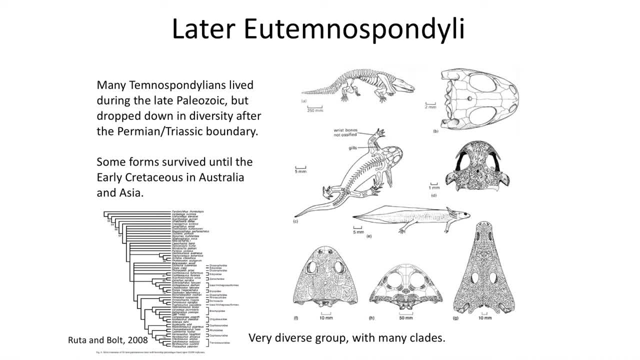 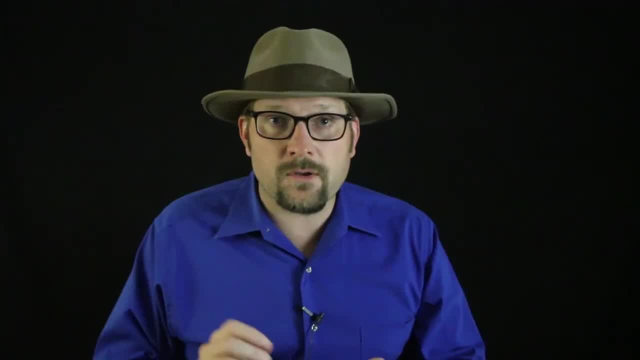 Including the Trimatosauria and the Caterpillar. These eutemnospondylans would survive in the Mesozoic, including the Trimatosauria and the Caterpillar. They hung on during the Jurassic with the last species known from the early Cretaceous. However, during the Triassic, within this group, modern amphibians including frogs, salamanders and caecilians, originated, and we'll talk about their evolution in a later lecture. Alright, let's now focus on the other major lineage of early tetrapods, the ones that 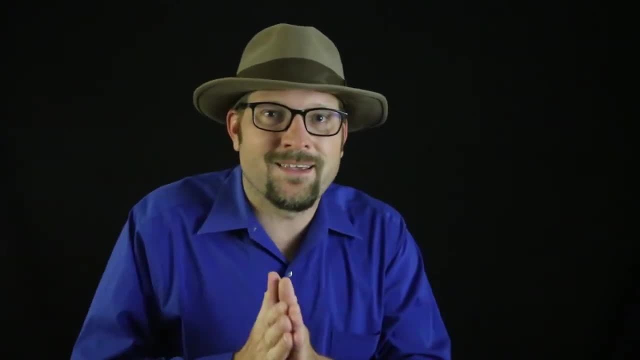 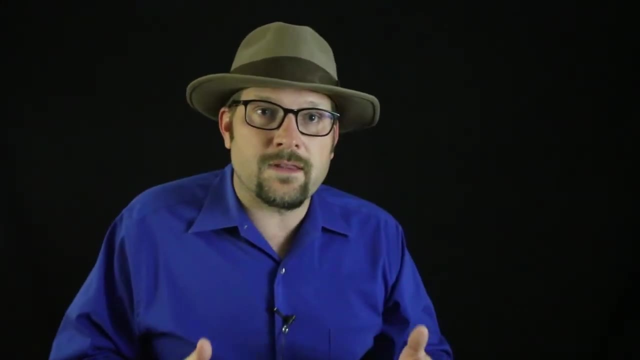 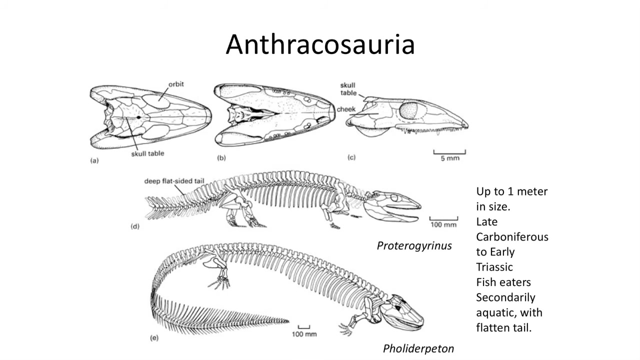 would eventually lead to reptiles, birds and mammals. These are called the Leptospondylans. The Leptospondylans are a diverse group that lived during the Pennsylvanian period and into the Permian. The early Leptospondylans are called the Anthracosaurs or Embolomera, which were elongated crocodilian-like. 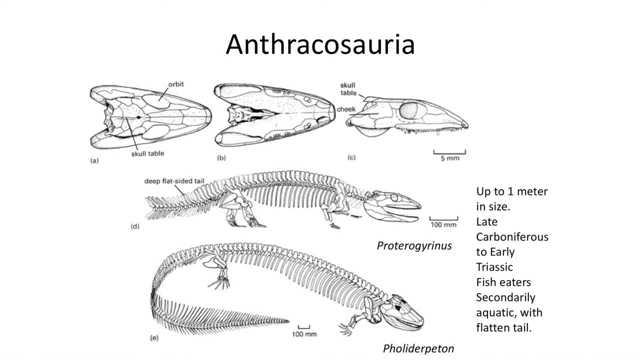 tetrapods. They grew to modest sizes and fed on fish. They were also known as the Leptospondylans. They were often fed on fish, although others were likely fed on insects and were more terrestrial in their habit. These Anthracosaurs lacked the open roof of the mouth of the Eutemnospondylans and had 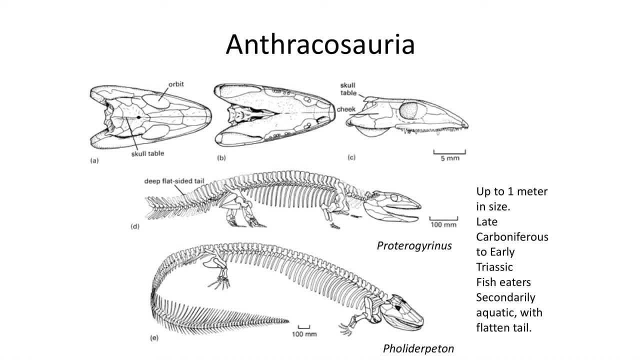 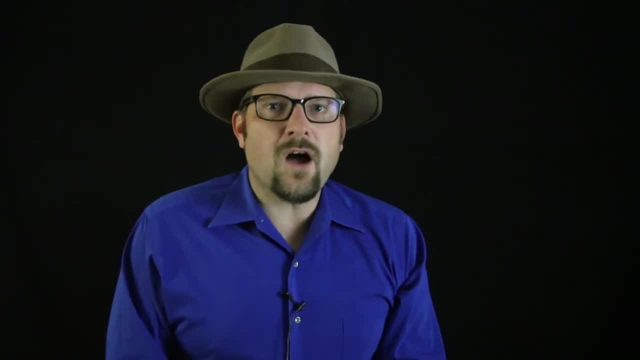 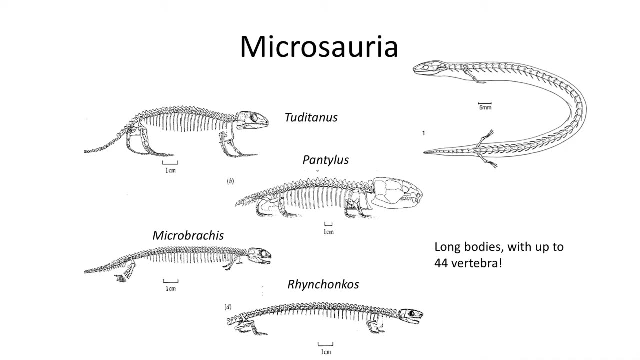 large eyes and a well-developed otic notch in the back of the skull for hearing. The next group of Pennsylvanian Leptospondylans are the elongated serpent-like Microsaurs, including the Cretaceous Microsaurs had numerous vertebrae between their limbs, making them long and tube-like. 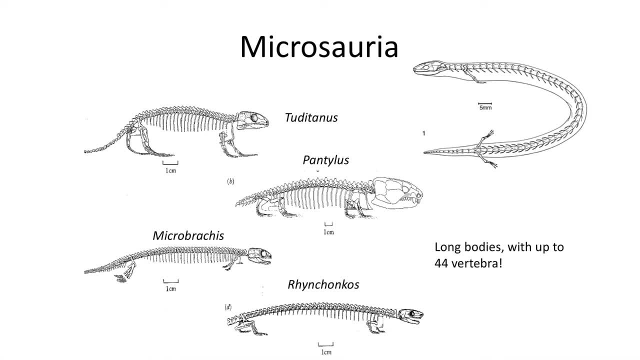 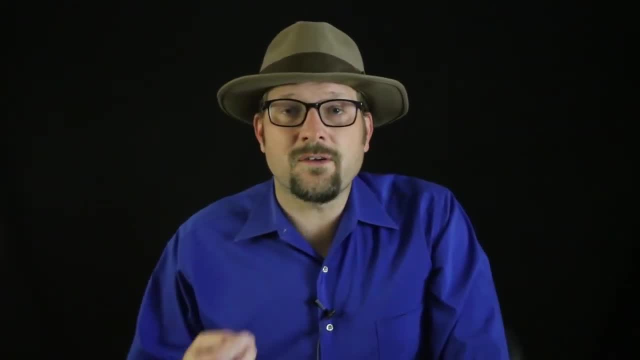 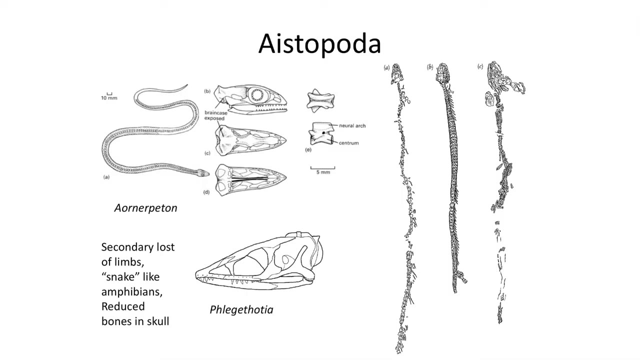 Microsaurs might not form a monophyletic group and their relationship within Leptospondylans has moved around lately. Several of the early Leptospondylans lost their limbs entirely, including members of the next group, Aesthiopods, which resembled snakes. 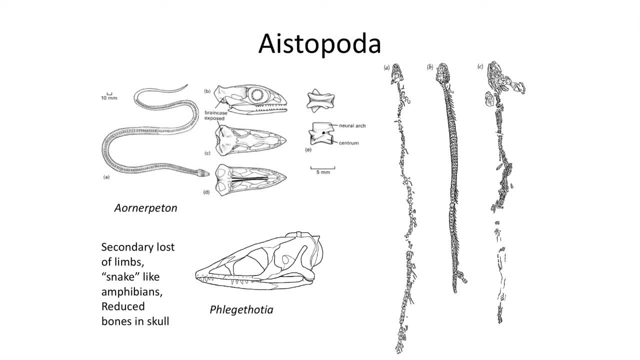 They have remarkably slender skulls which are very nimble and have the brain case exposed. These early snake-like animals likely took to the land and fed on the abundance of insects, And several got rather large in size with lengths up to a meter long, with 230 vertebrae. 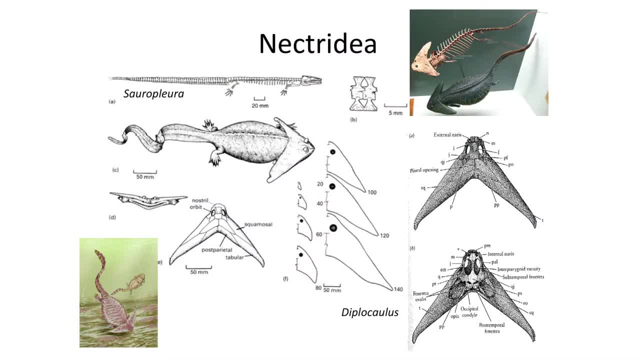 The next Leptospondylans are the Necrodendrons. Necrodendrons are the most common species of reptiles. They are the most common species of reptiles, The Necrodiae, the boomerang-shaped early tetrapod known from the Pennsylvanian and Permian. 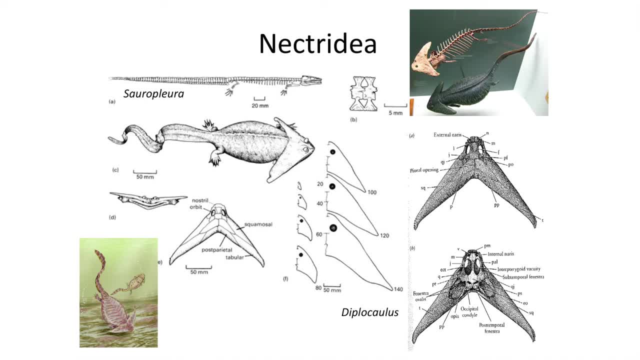 of Ohio and West Virginia, as well as other sites in Africa. The Necrodiae feature horned skulls that grew throughout the life of the individual, which formed long projections on either side of the head. These Leptospondylans likely used these horns to generate lift as they soared. 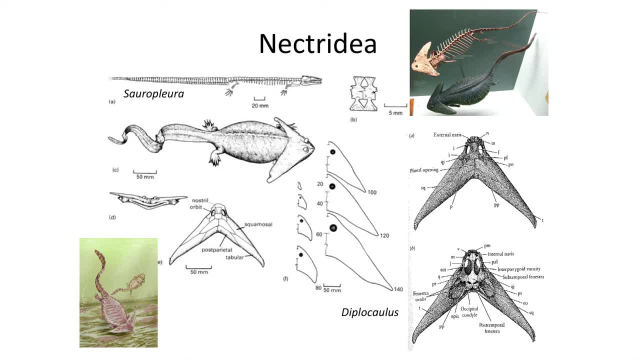 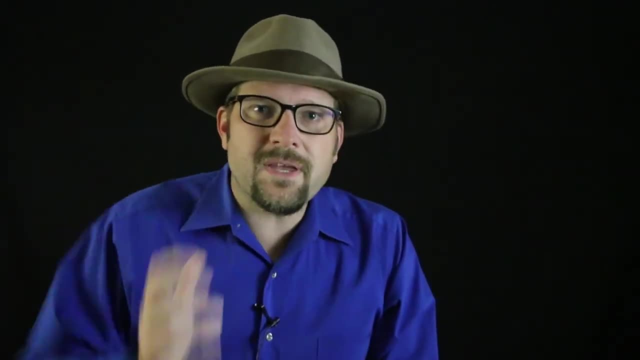 As they swam like wings of an airplane. These were likely fully aquatic early tetrapods feeding on fish and small aquatic invertebrates. The next two groups I'll mention are restricted to the Permian period and represent the biggest shift toward a more fully terrestrial lifestyle. 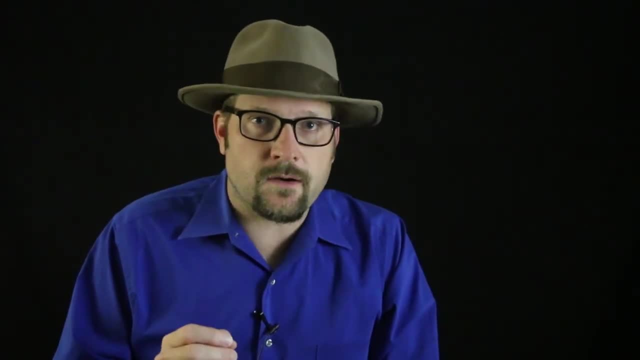 These two groups have shuffled around in their relationship to each other, but both are unique in having more upright limbs and better legs. The Necrodendrons are the most common species of reptiles. They are also known for their spiny, sharp, sharp limbs and better developed hands and 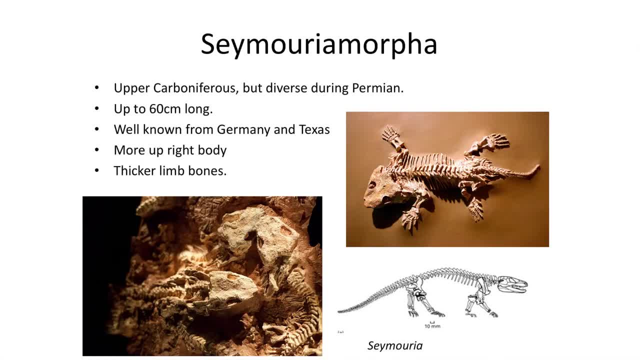 feet. The first group is the Seymoura morpha, a diverse group that is well known from some amazing fossil sites in Germany as well as in the United States. Several groups persisted in Russia into the Triassic. The genus Seymoura featured an upright body and thicker limb bones to support a more fully 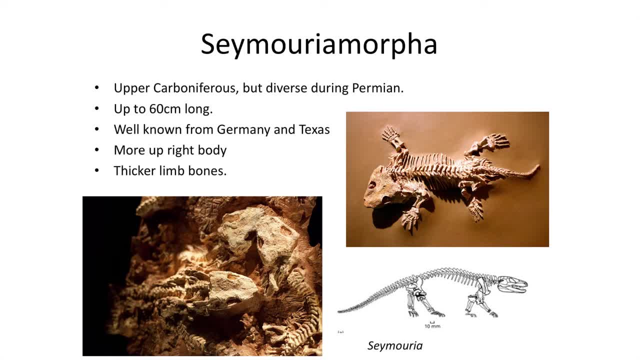 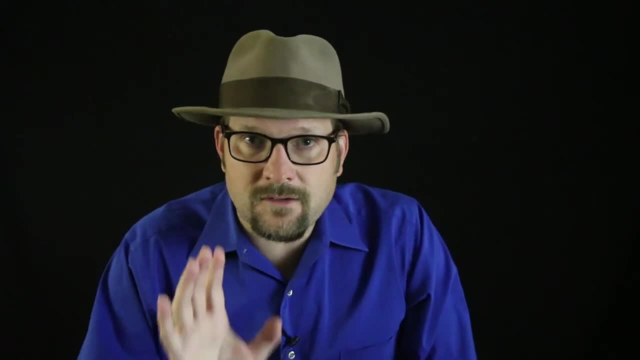 walking style of locomotion. The body was short and squat- squat and likely walked with an undulating pattern of limb movements, but had a shorter trunk than we have seen before. The last group of Leptospondylans are the most advanced of these early tetrapods known.